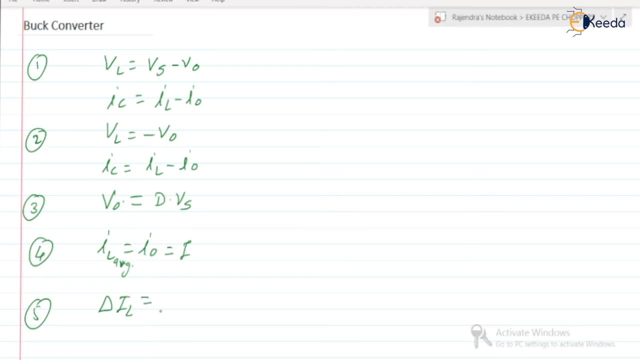 Yes, ripple in inductor current, So it is a delta. IL is equal to VS by L Into 1, minus D into DT. No need to memorize the expression, So please be careful. Next, how to simplify the numericals without memorizing the expressions. 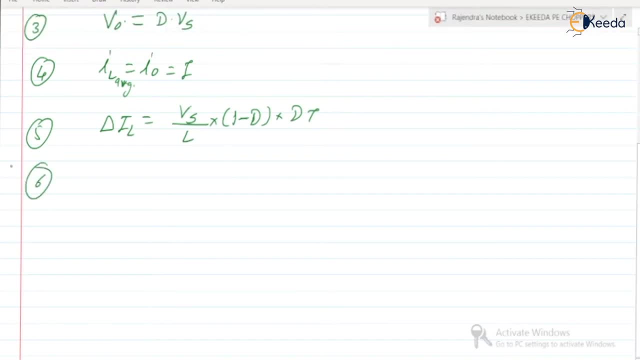 We will discuss. Sixth one is the IL max. Yes, what is the IL max? If you check axiom value of the inductor, current IL max is equal to. Is equal to Current load, current I plus delta IL by 2.. 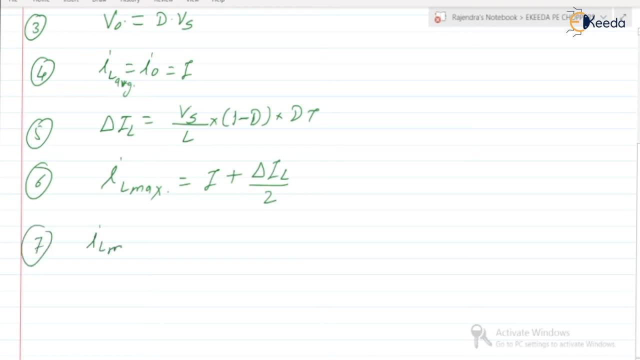 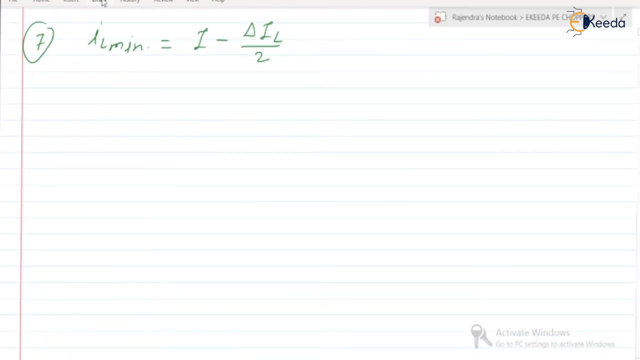 Okay, Similarly, IL min we are having. Minimum value of inductor current is equal to what I minus delta IL by 2.. Okay, This is the seventh one, Right. Next, what about the eighth? If you check the eighth, 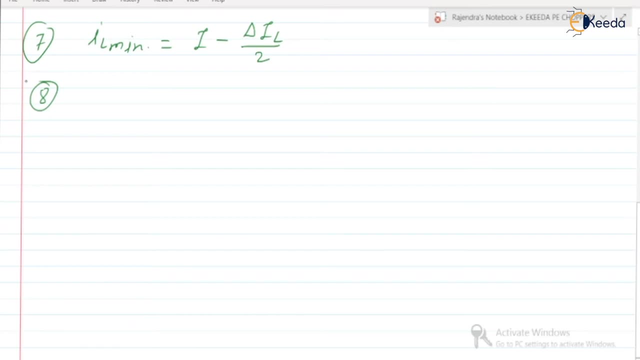 Yes, in the eighth, It is a source current. Okay, Source current Is: We have derived it Is is equal to D into I0 or D into I Right, D into I. Okay, This is like a average value only. 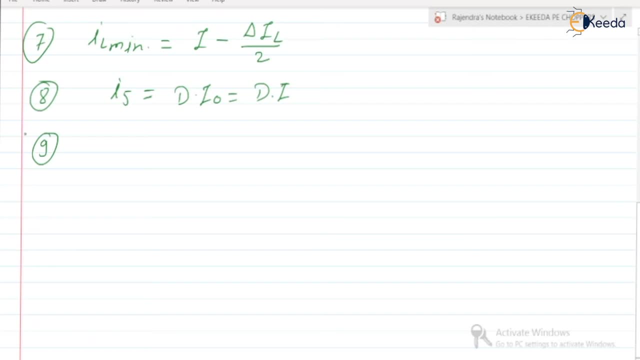 Ninth, it was switch current average and RMS. Okay, So we have derived it Is W. average is equal to what It is a D into I0.. Which is equal to D into I0.. Which is equal to D into I. 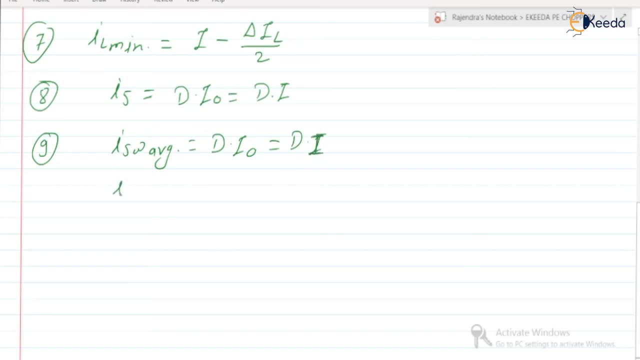 Okay, Load current Right. So next, What is the ISWRMS? ISWRMS is equal to under root D into I0. Which is equal to under root D into I. Okay, Tenth Diode current Right. 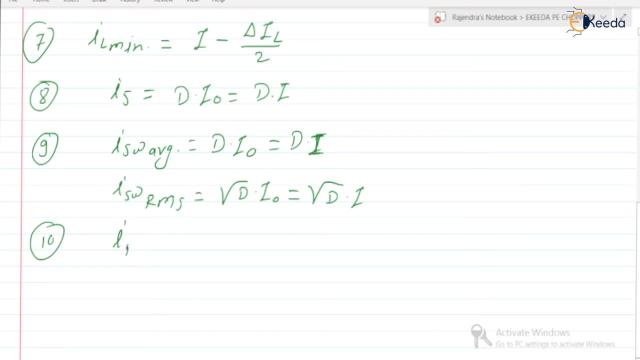 Diode current average and RMS ID Average. If you check ID average, It is equal to Diode current. Right Diode current. It is equal to 1 minus D into I0.. Or 1 minus D into I. 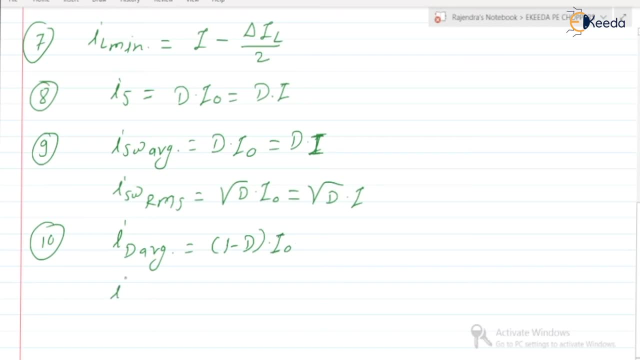 ID RMS Is equal to what It is: a Under root 1 minus D Into I0.. Or under root 1 minus D into I. Okay, This is about the tenth Right Next Eleventh. It was. 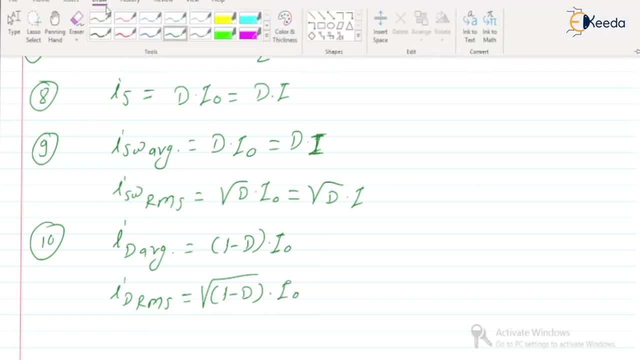 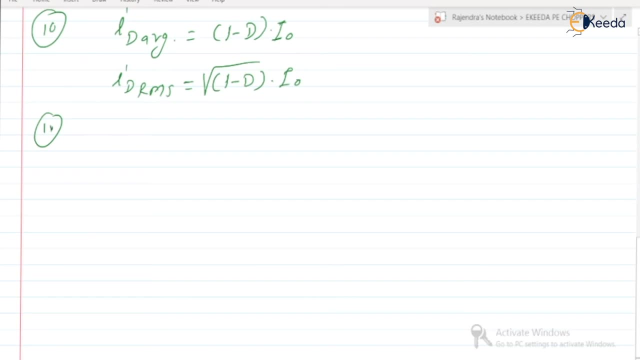 Yes. If you check Eleventh Ripple in capacitor voltage: Okay, This is about the tenth, Right, Next Eleventh, It was Yes. If you check Eleventh Ripple in capacitor voltage: Okay, Ripple in capacitor voltage. 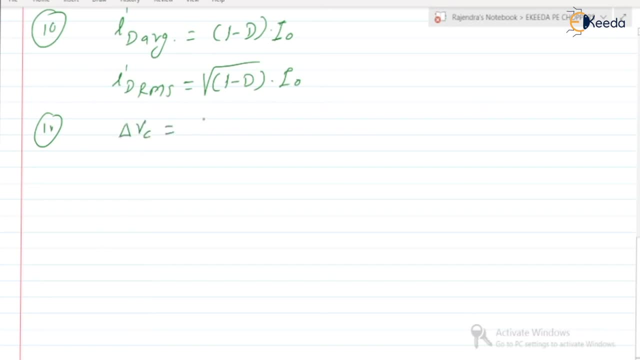 So delta V C, Delta V C. You have derived it. It is a V S into 1 minus D Into D, T square Divided by 8, LC, 12. D, at which Ripple is maximum Right. 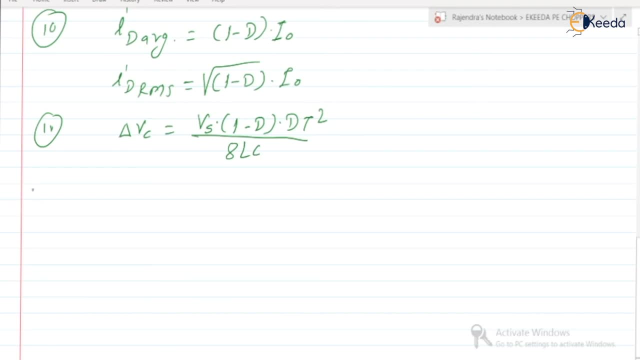 D At which At which Ripple is maximum. What was the value of that? D At which Ripple is maximum? Right D At which At which Ripple is maximum. What was the value of that D? 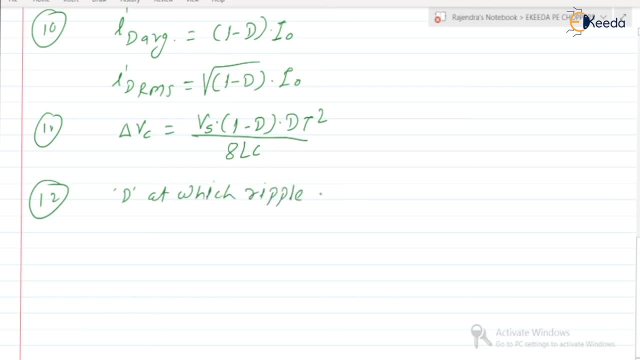 What was the value of that D? D At which Ripple Is Maximum? Yes, Is equal to How much It was, 0.5. Or 50%, Okay, Thirteenth Critical inductance. 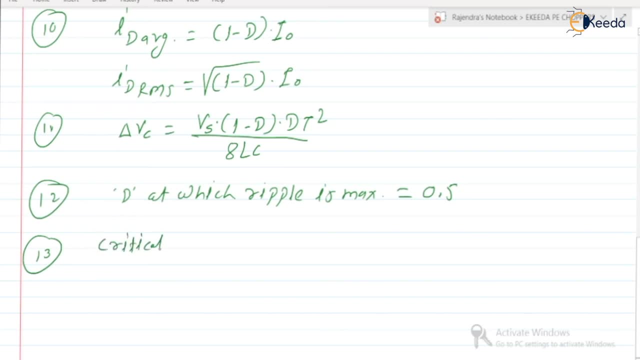 Critical inductance. Critical Inductance Right Is equal to What L Critical D At which Ripple Is Maximum? Yes, It is equal to 1. Minus D Into. 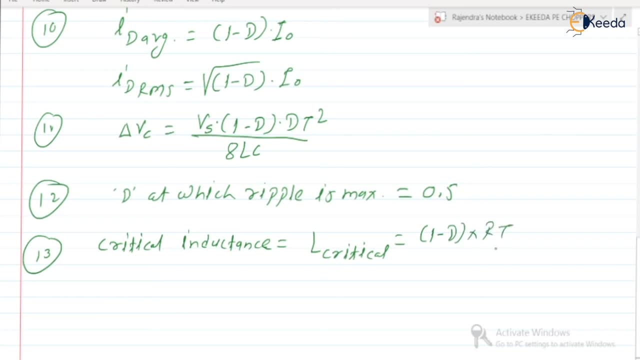 R Into T Divided By 2.. Okay, And Fourteenth Was C Critical Right, C Critical, That Is, A Critical Capacitance Equal Capacitance. 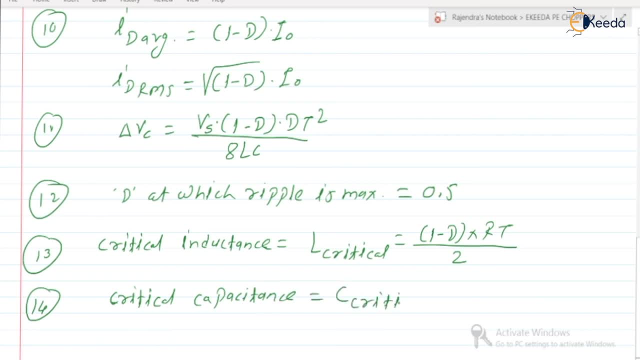 Right, So It Is 1. Minus D Into T Square, Divided By In L. Okay, So These Are The Fourteen Parameters Related To The 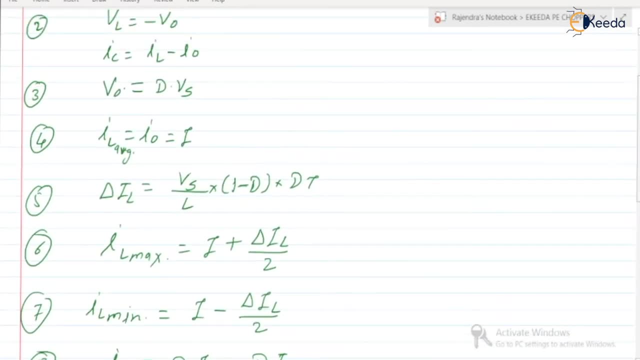 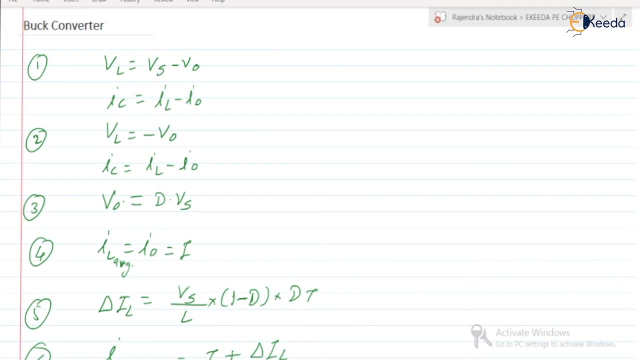 Buck Converter. Okay, No Need To Memorize To Discuss Numericals Related To The Buck Converter. Thank You.